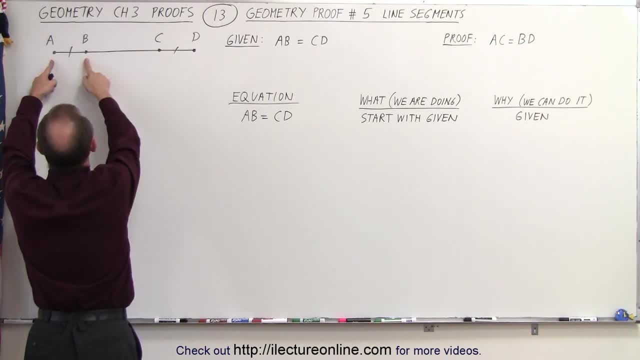 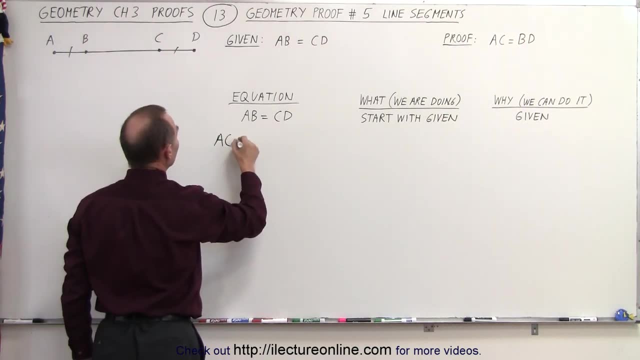 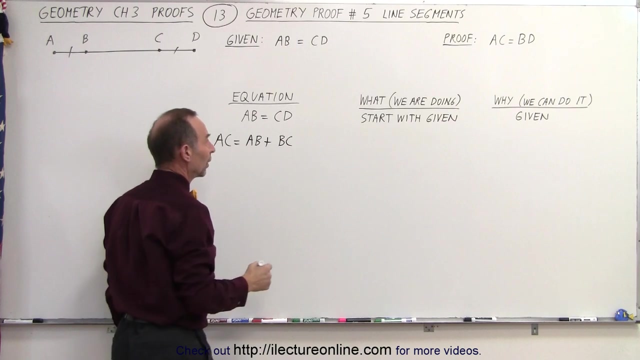 Well, AC here looks like it's the sum of length AB plus length BC. So let's do that. Let's write that the length from A to C is equal to the sum the length from a to b plus the length from b to c. so what we do here is we have segment addition. 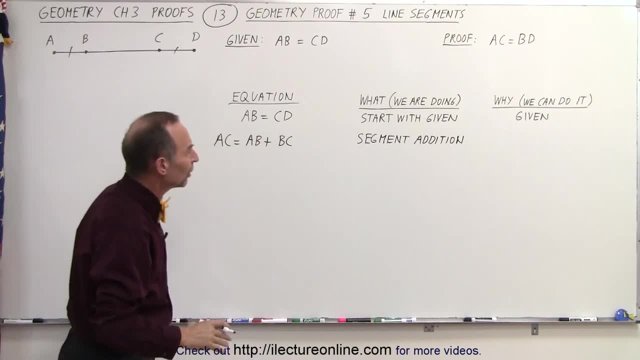 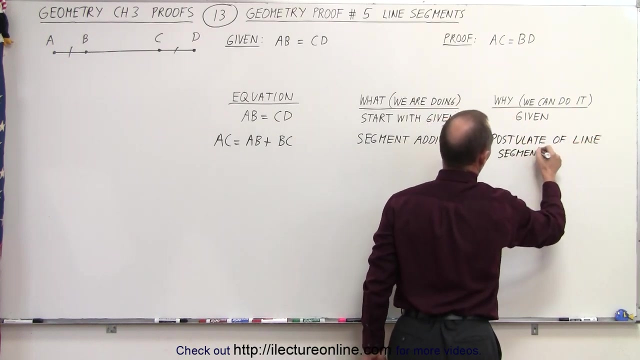 addition. now, why can we do that? well, there's a postulate that says that if we add two adjacent line segments, that they add up to the total length. in other words, we can do this because we have a postulate of line segment addition, which means that we can make a valid claim. 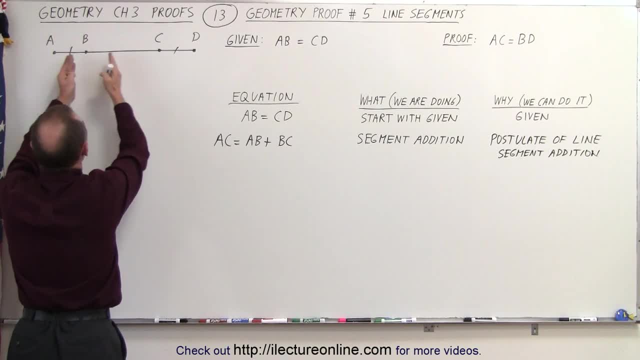 that we can say that the length of a, b plus the length of b- c is the length from a to c, because that's self-evident. that's what we mean by a postulate. we don't have to prove that. we can simply see that it is self-evident that the sum of those two must add up to a- c. 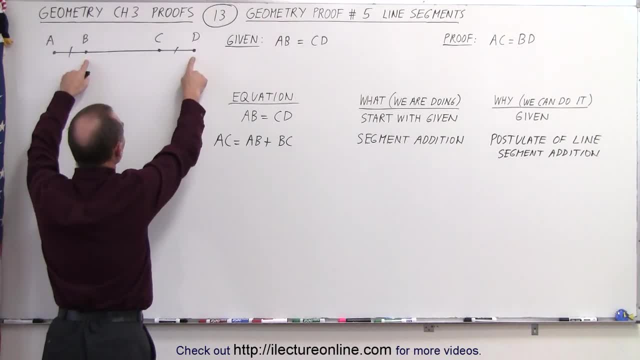 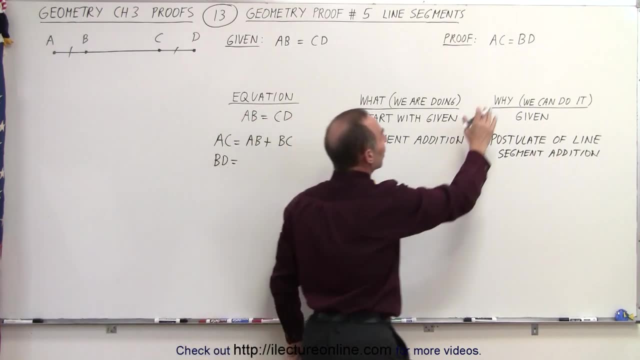 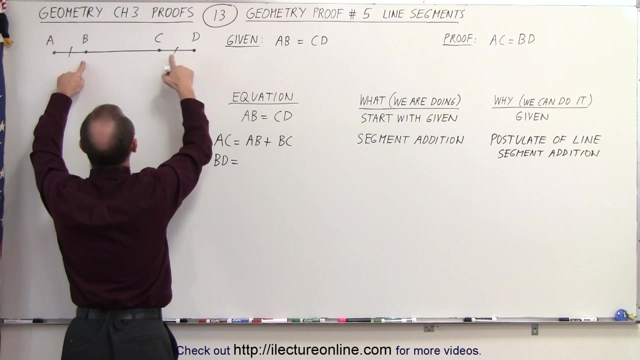 we can do the same thing for the segment from b to d. we can say that the segment from b to d- and why would i pick the segment from b to d? because that's part of the equation of my proof. so i can do the same thing here. i can say that the segment from b to d is equal to the segment from b. 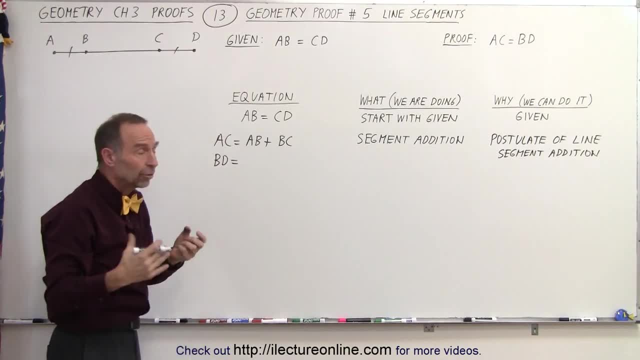 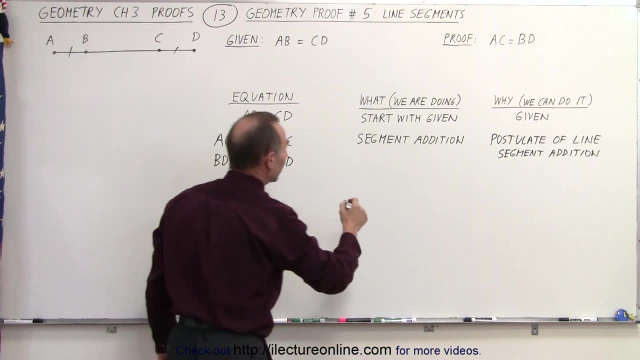 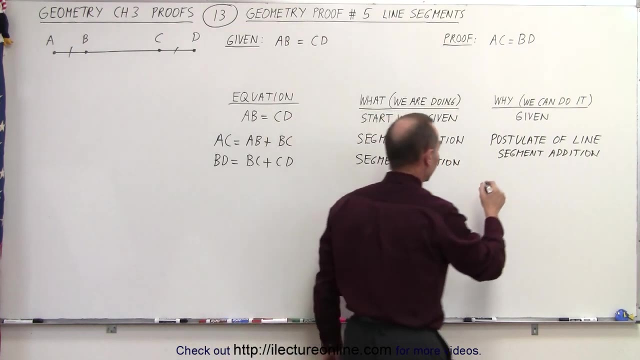 to c, plus the segment from c to d, at least the length of those segments. so this is b c plus c d. again, i can do that, i can call that segment addition and the justification is again the postulate of line segment addition. hmm, what do i do next? 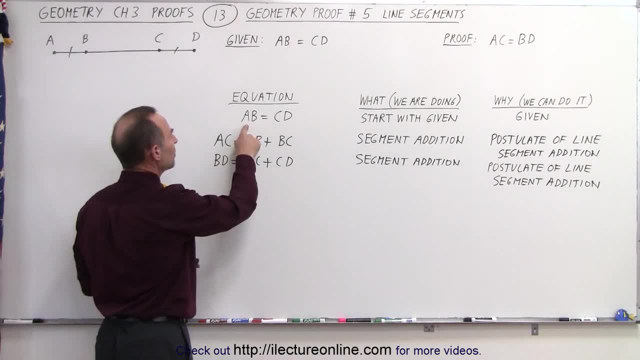 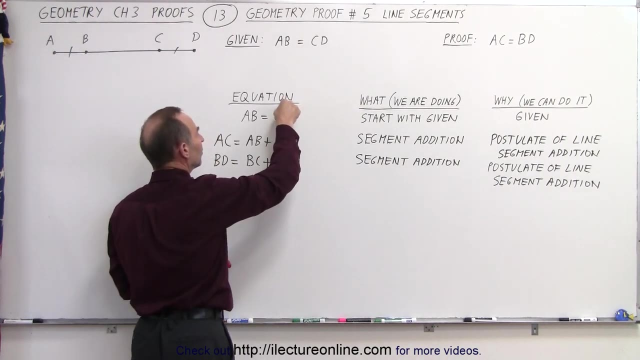 well, let's see. here i have an equation that says that a- b equals cd, meaning i could take this cd and replace what cd is equal to aha. i think that's a good place to go next. so here i see that this cd is equal to this cd, which means that cd is equal to a- b. i can make.